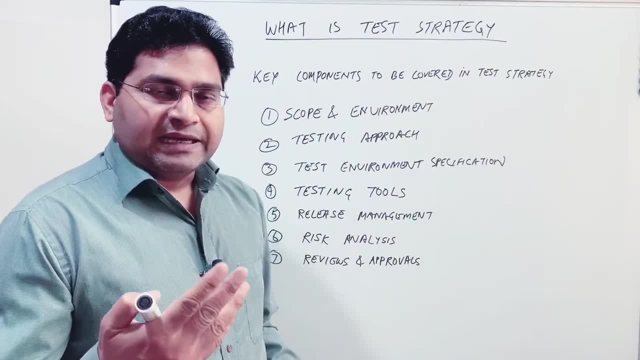 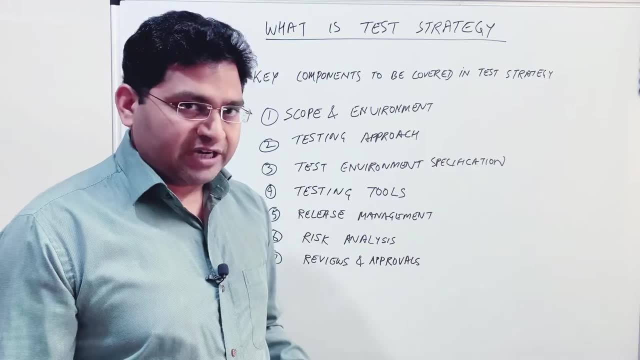 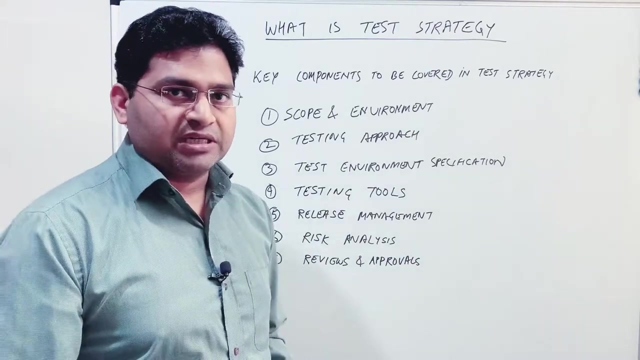 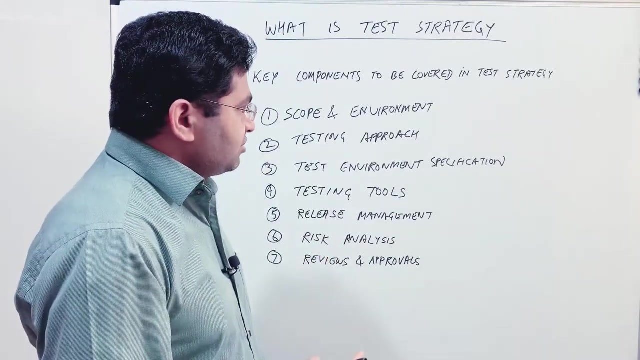 you know, testing document And like test plan is a document, So test strategy is also a document, which is, which can follow a predefined template. But if you see on my screen, these are the key sections that you know need to be covered as part of the test strategy document. there will be more sections as per needed by the organization, But these are, you know, like key sections that should be there And, if required, organization or based on. 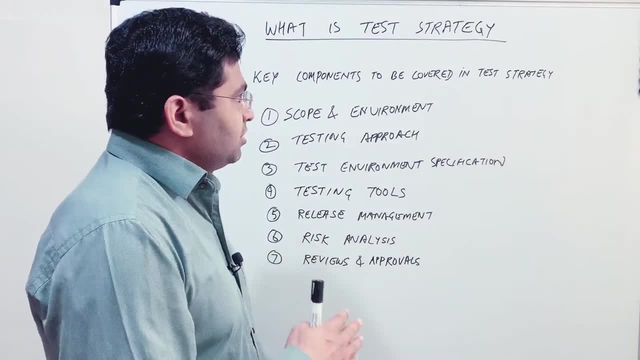 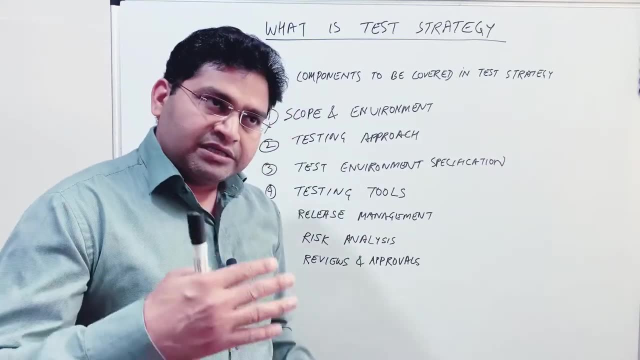 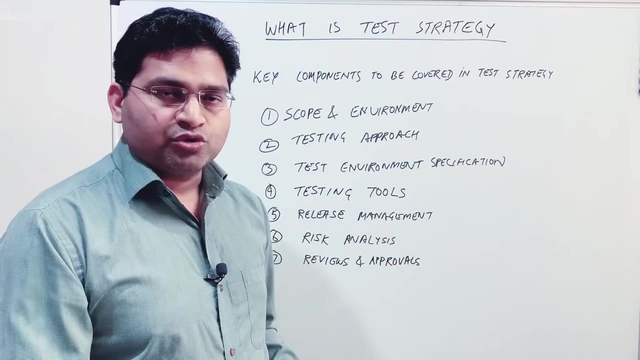 the needs of the organization, you can update the content of the test strategy document. Now, what exactly is test strategies, or test strategy defines the general way Testing will be approached within an organizations, so it is independent of the project. So, for example, 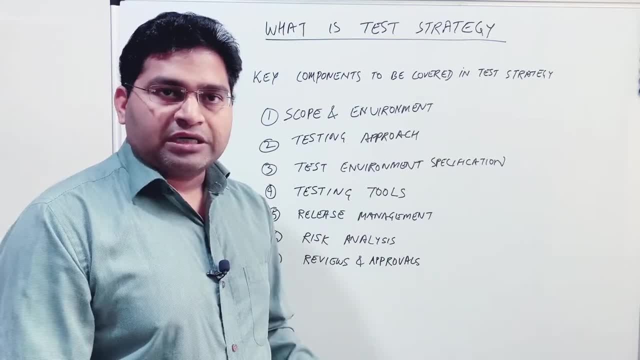 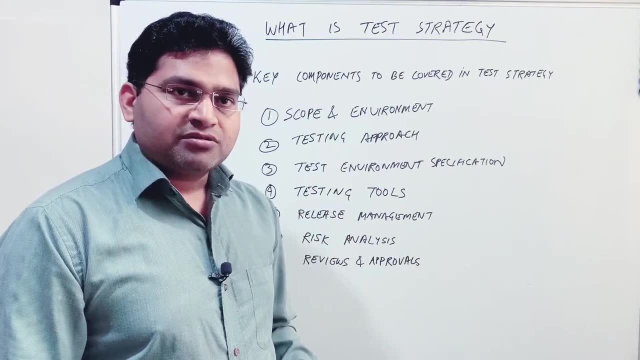 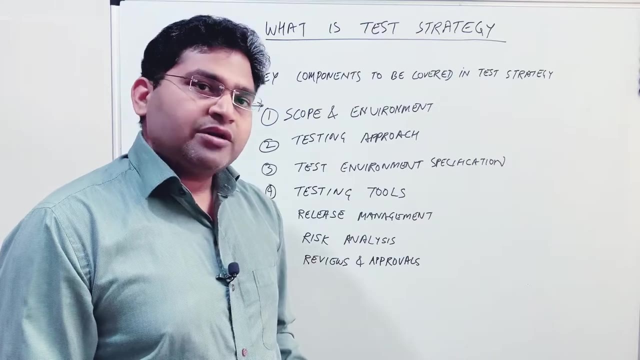 there is an organization, say you know big organization, IBM or any other big organization, and IBM wants to have you know o to define a strategy document. So IBM, as an organization, will define a test strategy document which will be independent of any specific project. What this means is that it will be very high level. 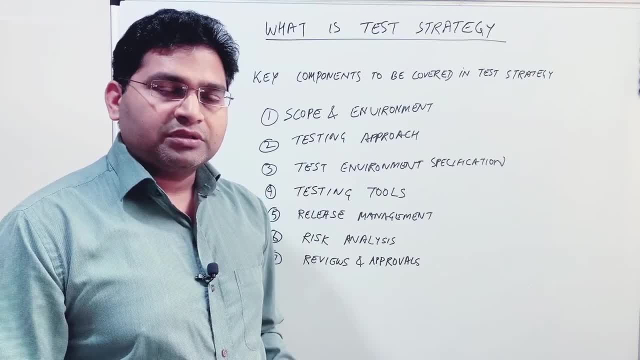 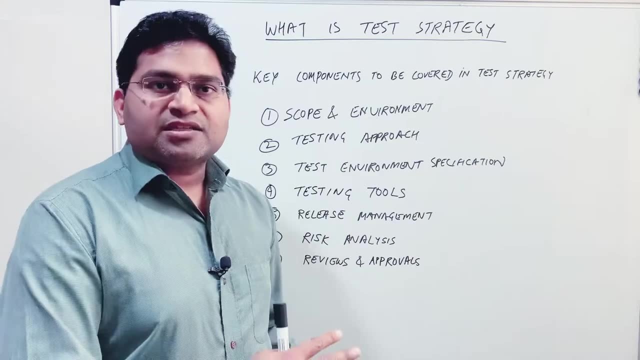 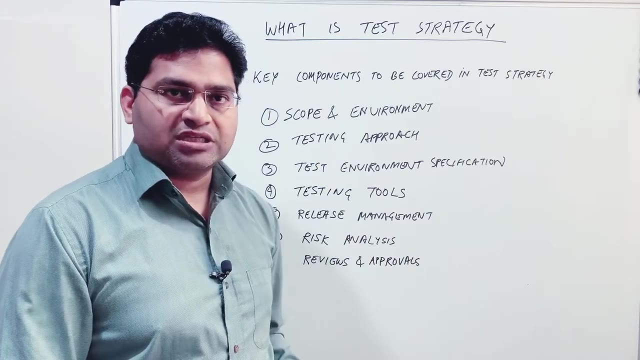 and it will cater for, you know, the key things or key approach that needs to be followed by any testing project that will be, you know, performed within the organization. Doesn't matter what type of testing project it is. The strategy will outline the high level approach of testing. 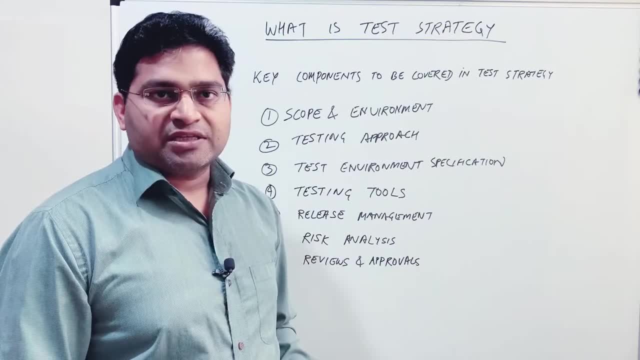 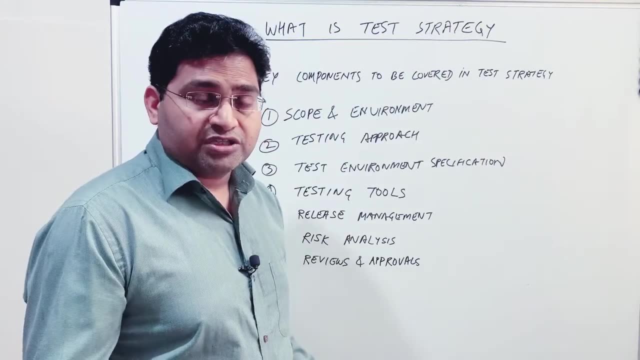 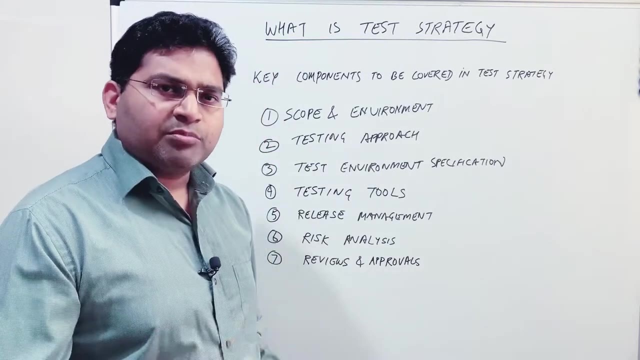 and other related activities of testing across the organization. All right, so this is basically, you know, high level definition of test strategy. It is at the organization level and it and then also depends. So I'll cover a couple of more details. Sometimes test strategy, if there is. 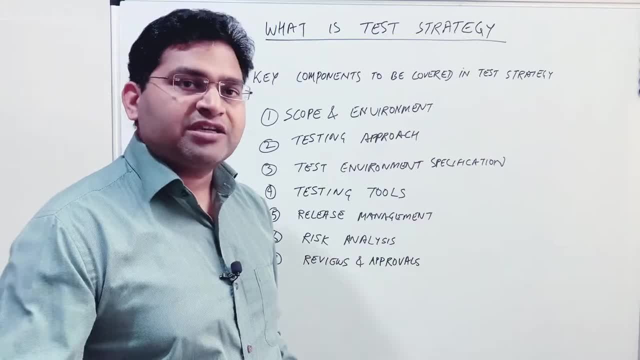 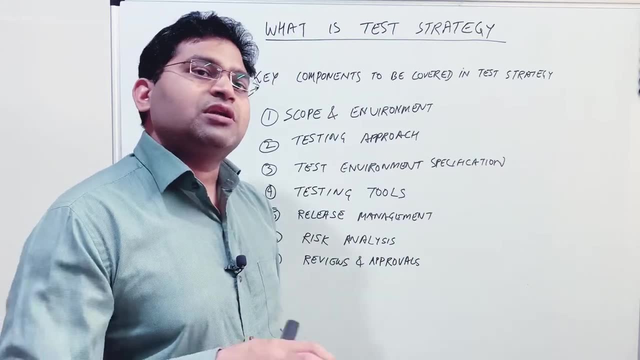 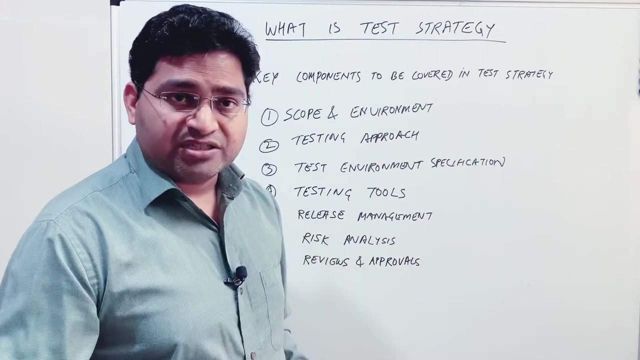 you know, like a small organization with just one project, there might not be two separate documents. So there might not be separate test strategy and test plan. So test strategy might be included within the plan itself, Okay. but if it is a big organization, there will be an organization test. 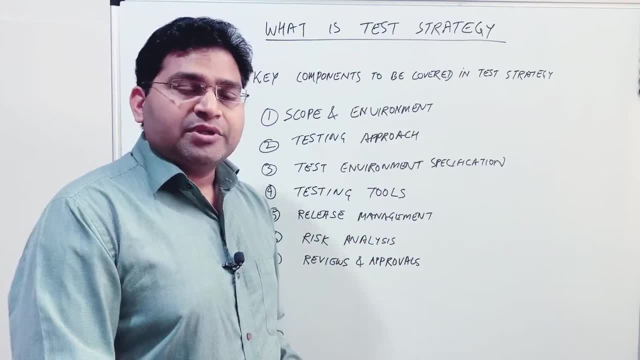 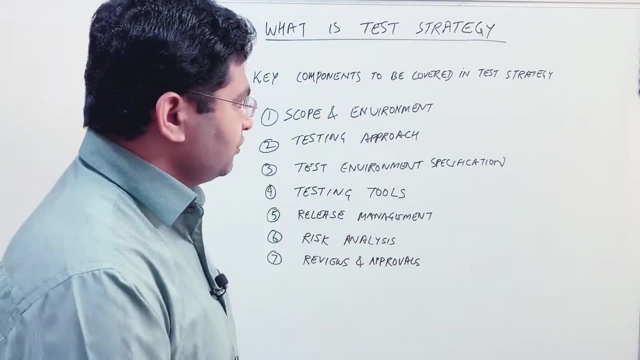 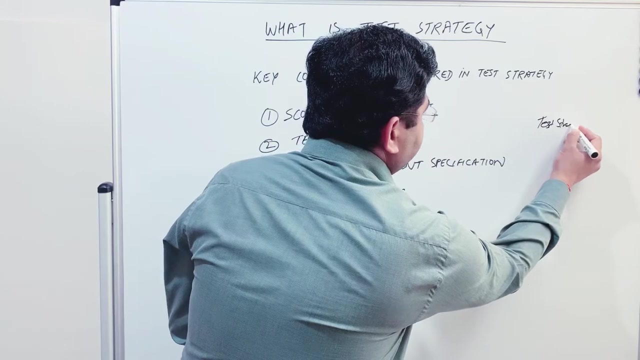 strategy document and then there will be multiple- you know test plan as per the project. So a separate test plan for each project, right? So if we talk about strategy and plan hierarchy, So you will have you know test strategy and then, below test strategy, you will. 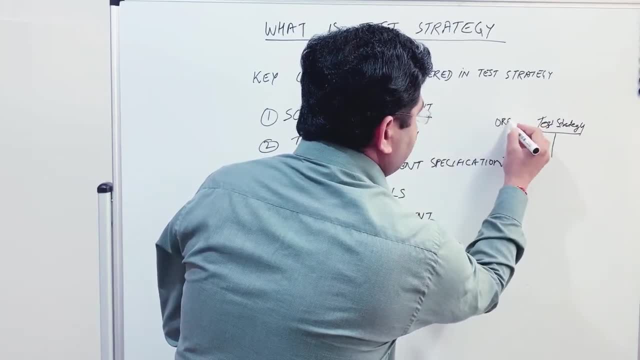 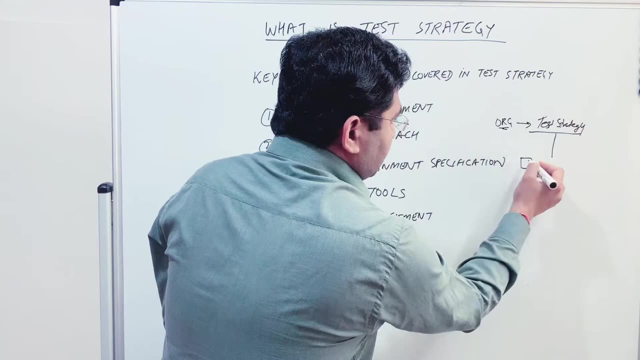 have, you know, multiple projects. So test strategy will be at the org level. So organization level will be defined if it is, you know, like a big organization, and then below the organization in the org chart you will have multiple projects. Say, for example, I have project. 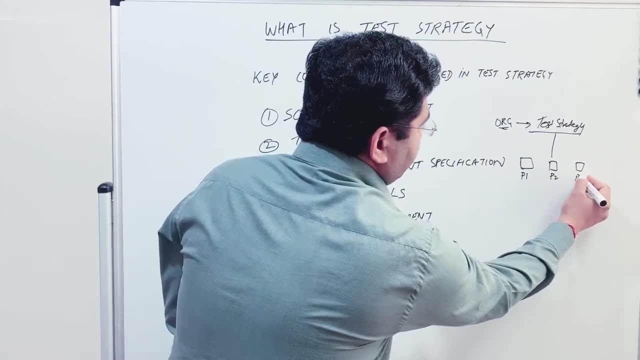 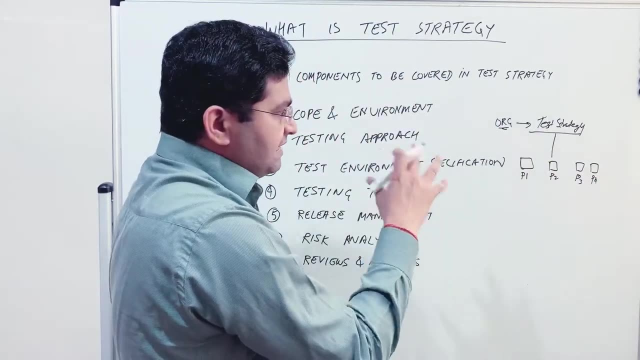 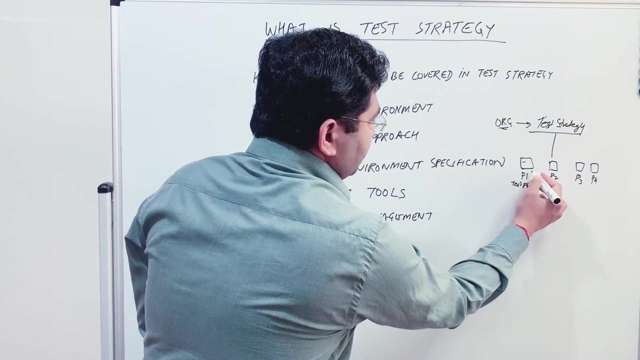 one, project two, project three and a project four. So many many projects. So any project that will be tested within that particular organization will have its own test plan right. So test plan will be specific to project and test plan refer to the high level testing approach that has been. 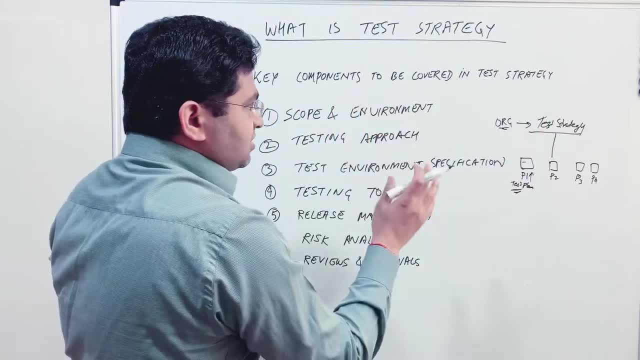 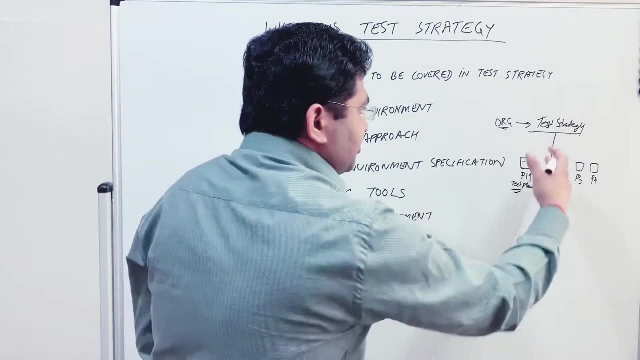 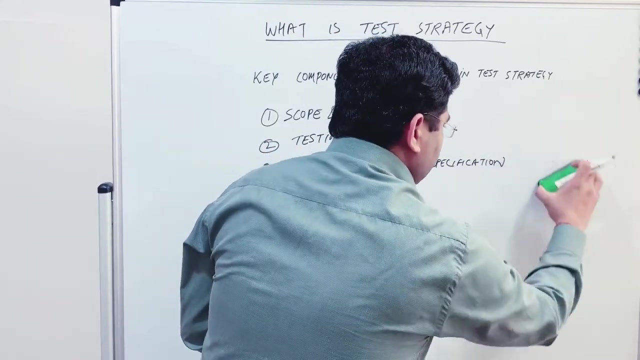 defined in the test strategy and they'll get most of the details from the strategy and try to align their software testing of the project as per the organizations test strategy. okay, So this is a broad overview of the test strategy and how it is related with test plan. okay. 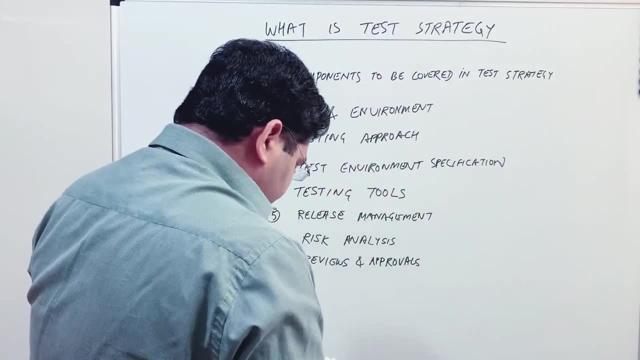 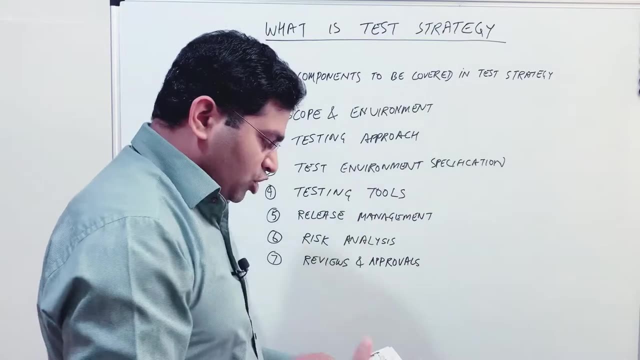 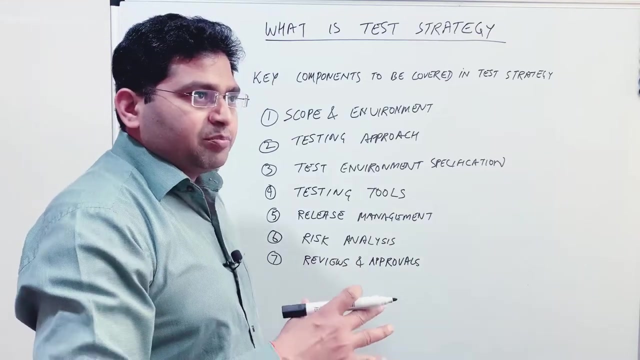 Now what exactly test strategy includes. It includes the details of test types, environment, you know, any artifacts that need to be produced by any of the project, the project. so it doesn't matter. a project a is doing testing, b is doing testing. the test strategy. 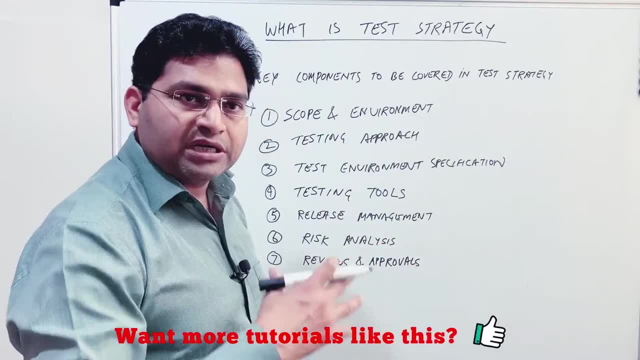 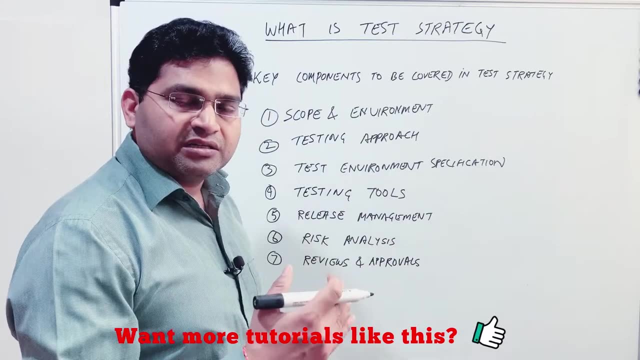 will define high level across the organization, that when you are doing or when you are engaging in testing of any project, these are the list of artifacts or these are the test artifacts that you need to produce right. so, for example, you need to come up with test summary report. you need to come. 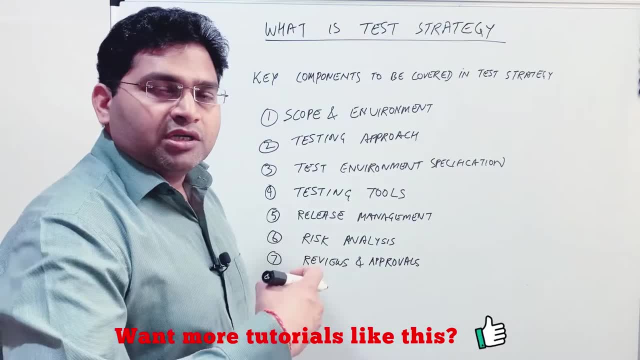 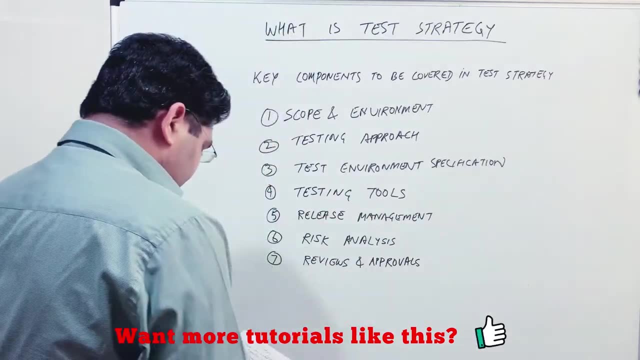 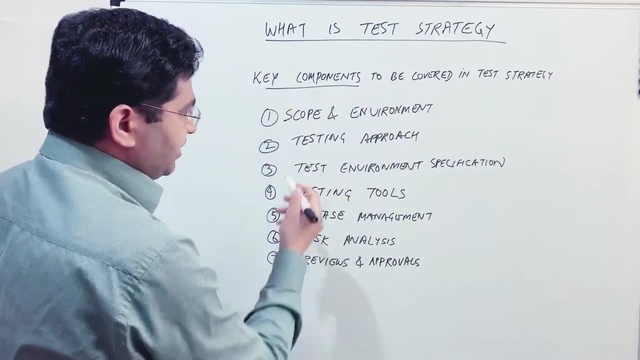 up with test plan for the project. you need to come up with the. you know test cases, right? so all that high level details goes into the test strategy. okay now if i talk about the key components of test strategy. so these are the seven key components that need to be covered. 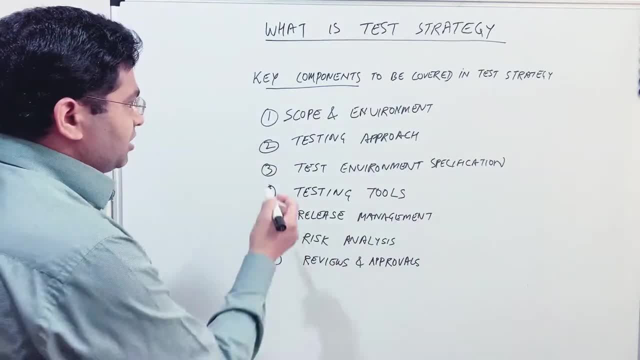 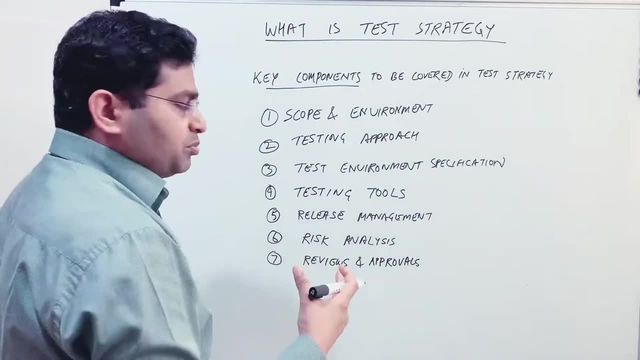 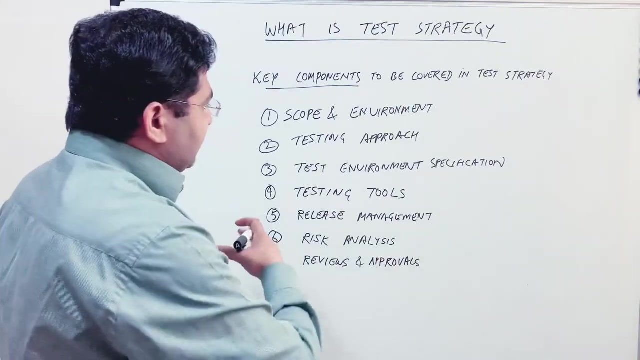 in the test strategy document when you are, whenever you are documenting, first thing is scope and environment. so what all you know scope should be considered whenever any project is being considered for testing or testing needs to be engaged in any you know project. so what is the scope and environment? 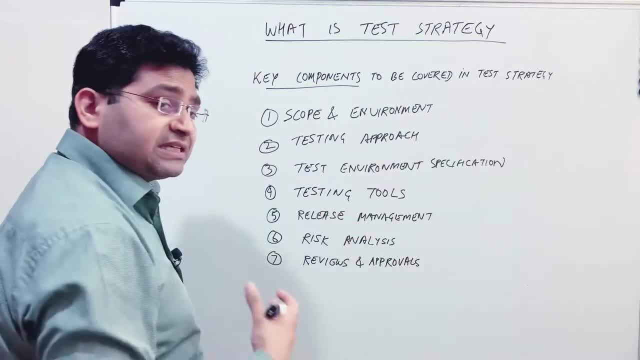 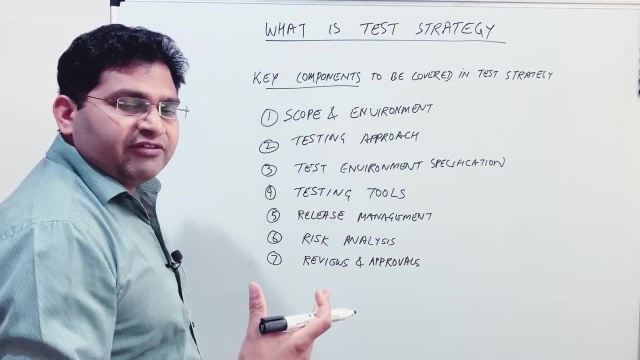 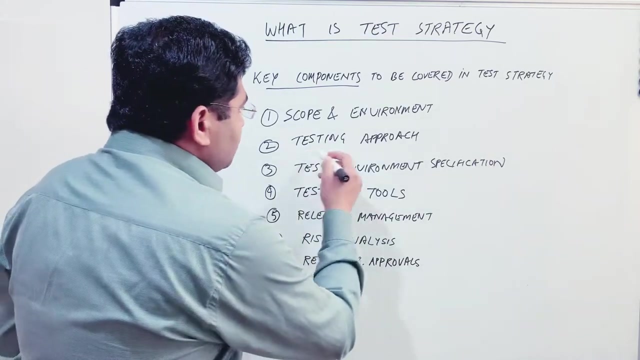 then you know testing approach, what all test levels need to be followed, say, for example, in the test strategy document, as at the organization level, i want to define that unit testing, integration system, system integration testing, user acceptance testing- all those testing levels need to be followed and within those testing level, what all details need to be followed. 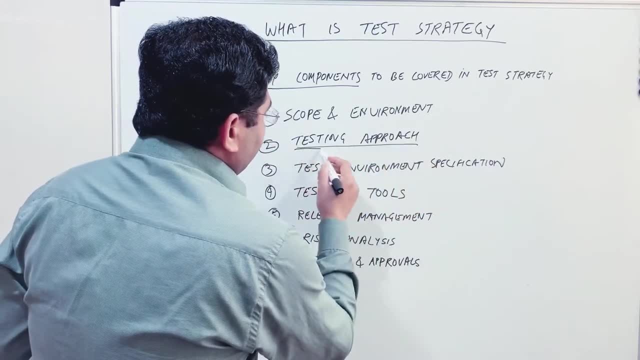 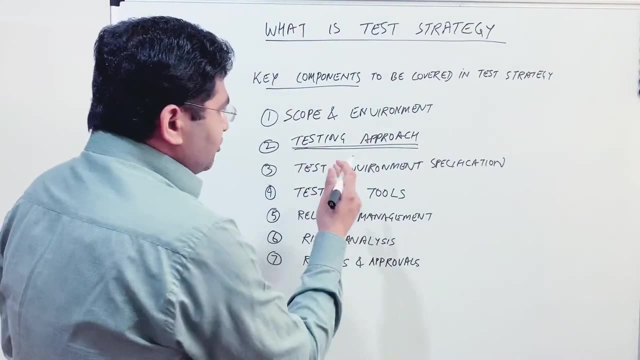 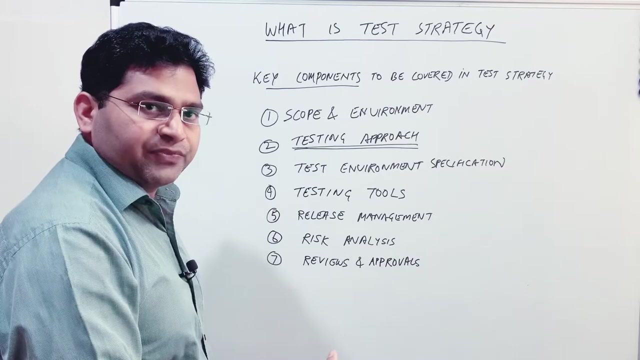 so, at the org level, testing approach will be defined and then, based on the project or type of project or complexity of project, this testing approach will be, you know, carried forward in the test plan and updated as per the project. okay, so it won't be copied, as is from the strategy, but it 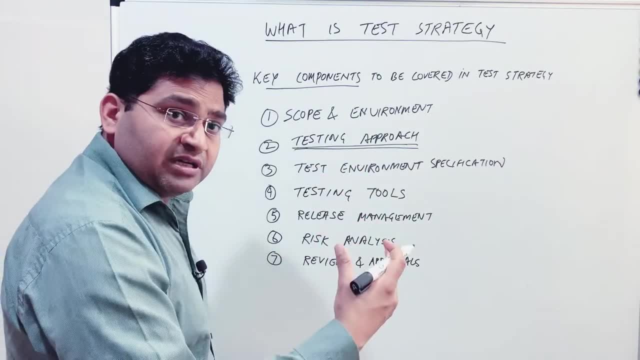 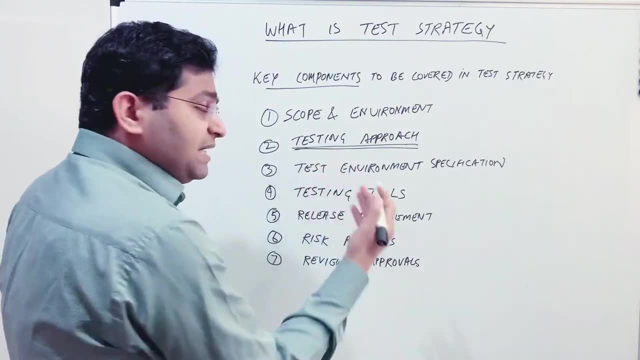 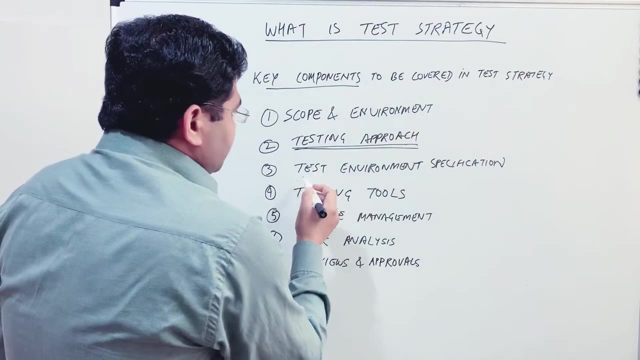 will be. you know, strategy will be referred and it will be a baseline for the approach in the test plan for a project project but and there will be an extension to the approach. similarly there will be an extension of scope and environment. then strategy will also consider about the test environment specification. 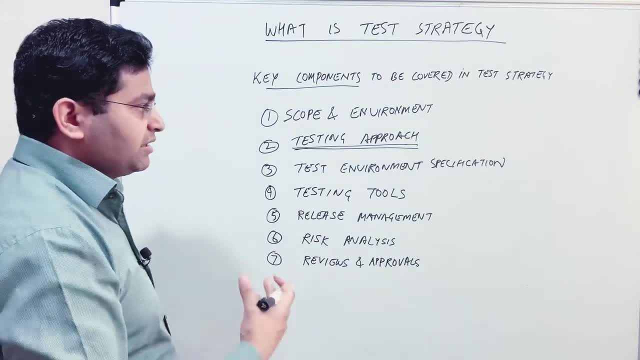 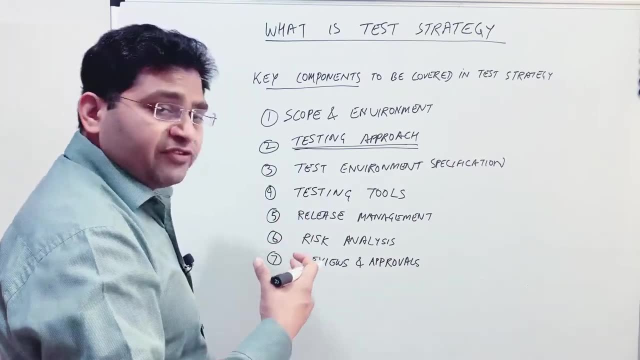 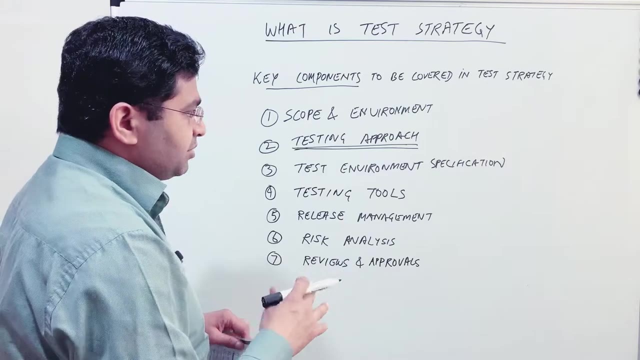 so what all test environment detail need to go there there, how the test environment will be spin up, who will be responsible? uh, what will be the specifications over the test environment? so all those details at the high level, at the organization level, right, say, for example, at the organization level, whenever we are engaging into testing or any project is engaging into. 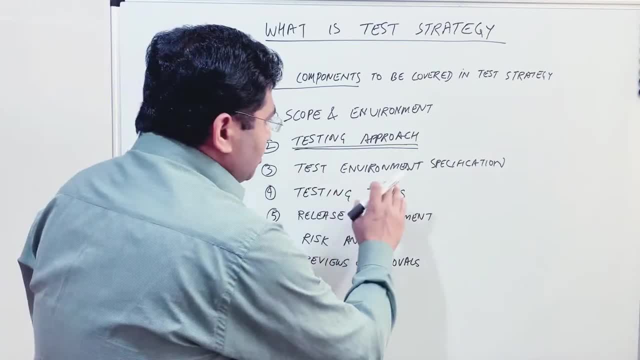 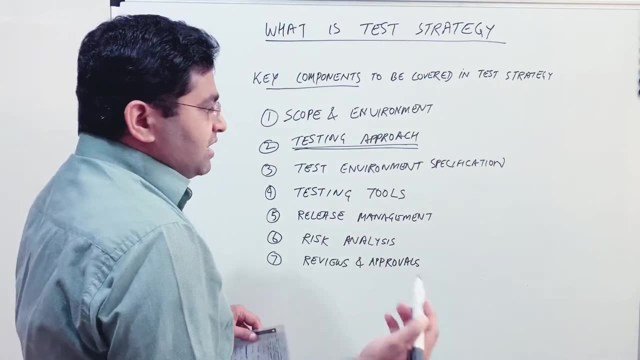 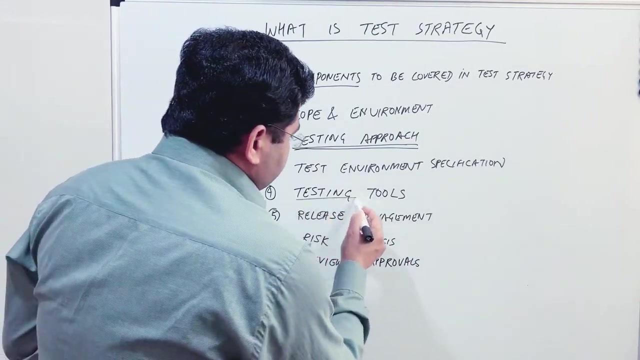 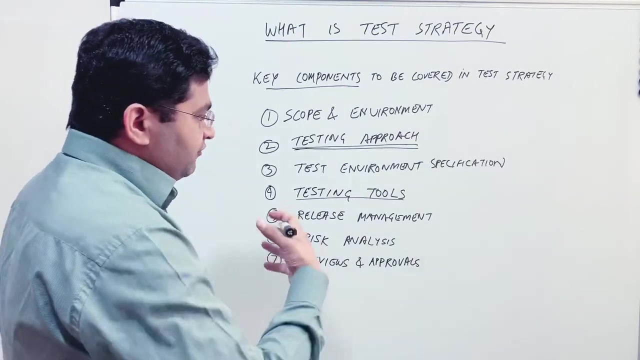 testing. they need to ensure that the test environment is as close as production environment. okay, so that could be one of the point in the test strategy. so a test environment specification needs to go there. at a broader level, then all the testing tools. so what testing tool will be used for test management, for defect management, if there is automation? that 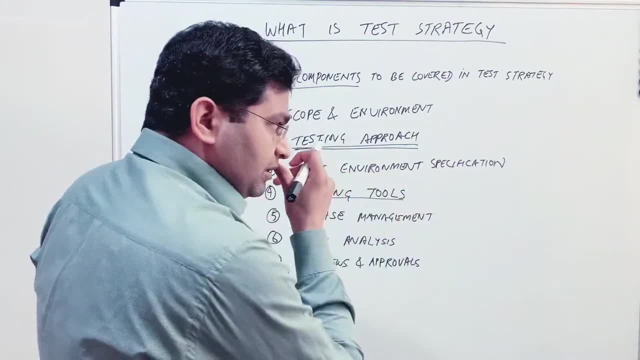 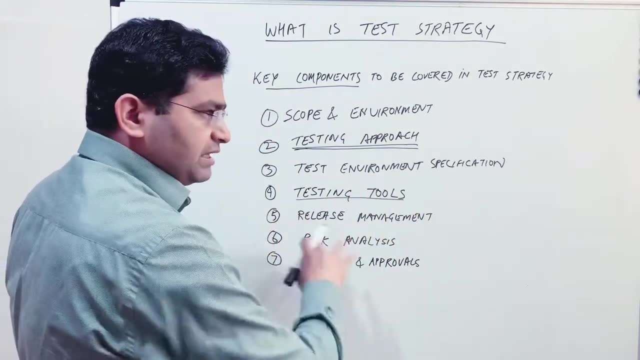 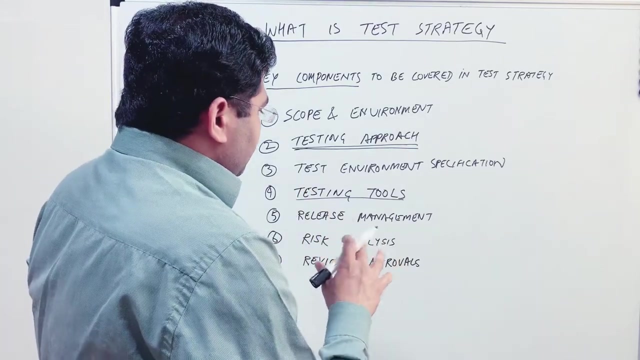 needs to be done, what all testing automation tools will be used. what this helps is in say, for example, on organization: with an organization there could be hundreds and hundreds of you know projects going on when you define the organization level test strategy and other you know high level test strategy. 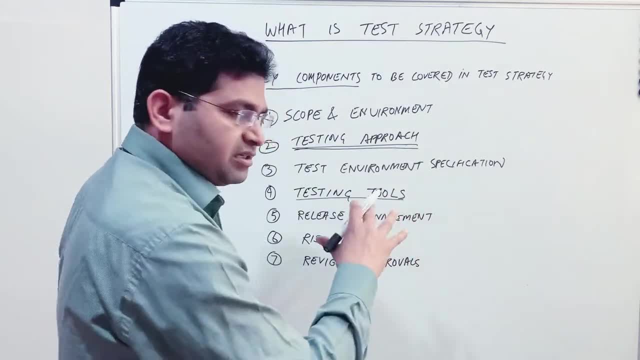 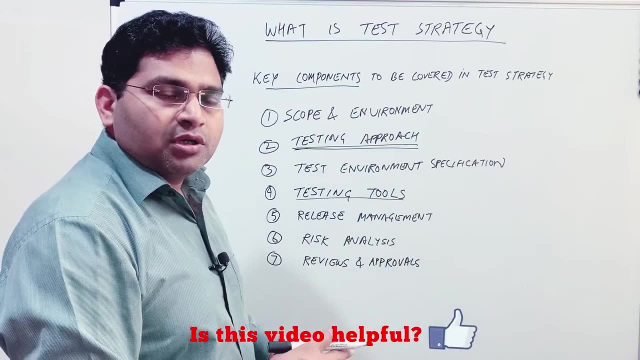 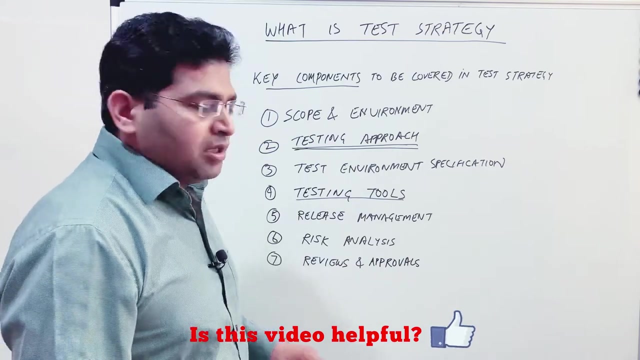 the testing tool tools. uh, and you define the testing tools, then there is a, you know, a bit of consistency across the projects, right, so there is no um confusion. say, for example, project a is using selenium, project b is using tosca, project c is using something else. so when you define testing tools and a list of 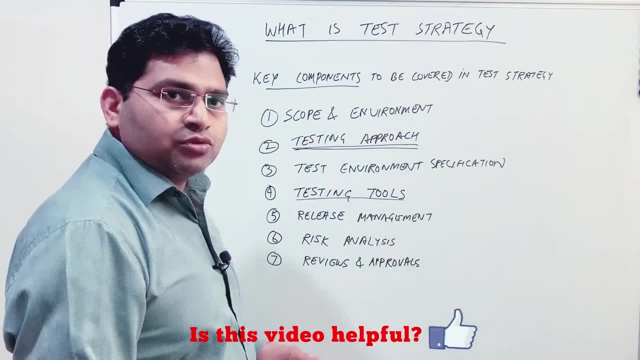 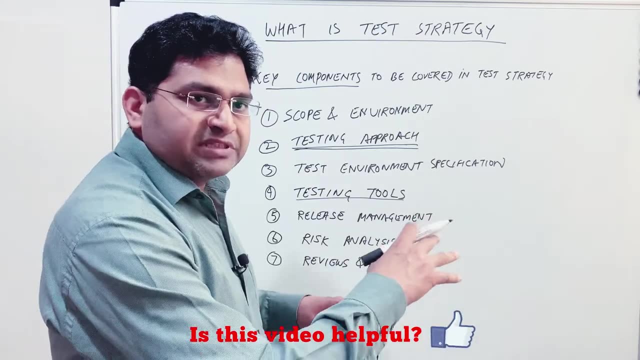 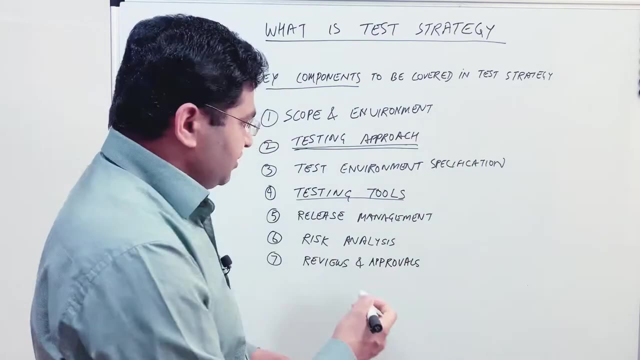 tools that can be used in the strategy. those are the tools that the team will use and they'll be maintained by some, you know, center of excellence or, um, some some central eyes team and that will help the other projects within the organization, uh, during the testing activities, right, so, um, the next thing is around the release management, how the builds will be. 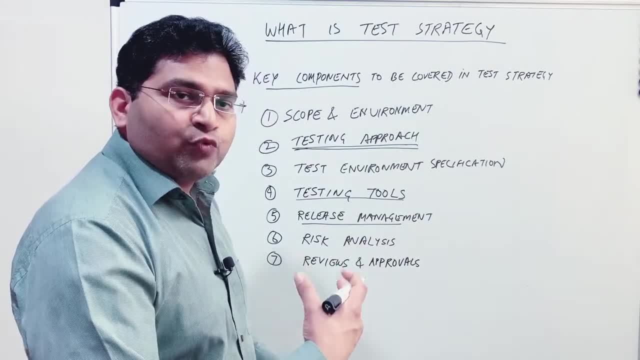 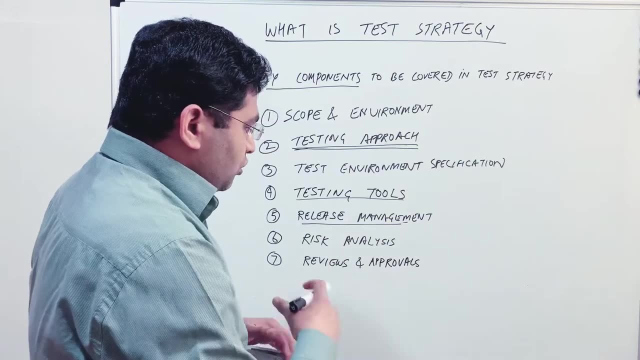 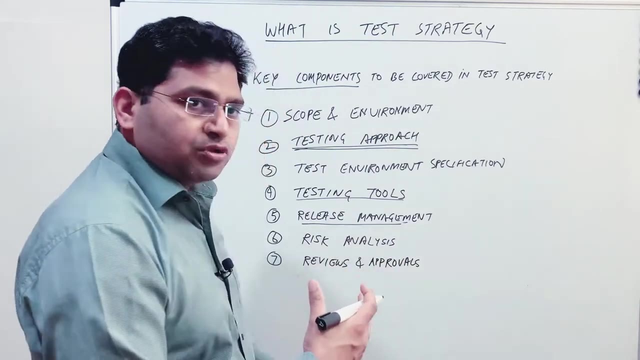 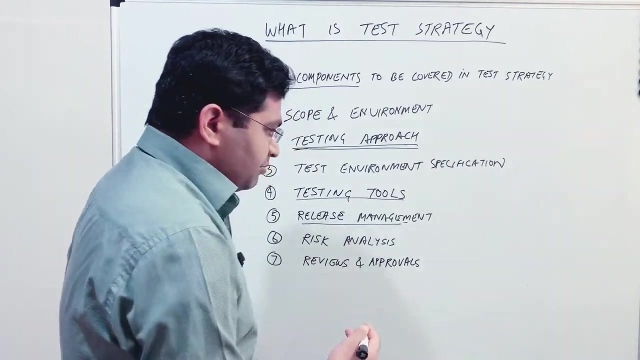 managed, how the release will happen to the testing. um, what will be the frequency of the build. all those details will go into release management section. then risk analysis- uh, what all projects need to consider about when doing the risk analysis of the project. and reviews and approval. who all will be reviewers or approvers in any project? say, for example: um, if i am a project a. 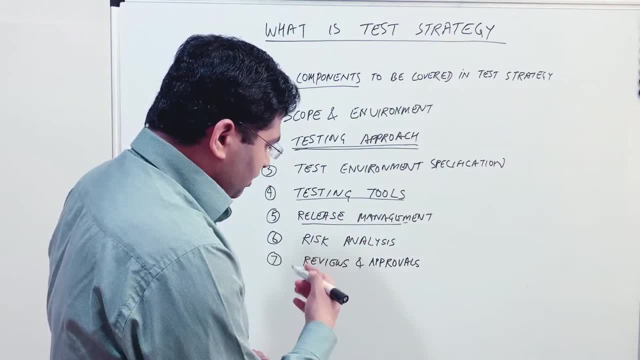 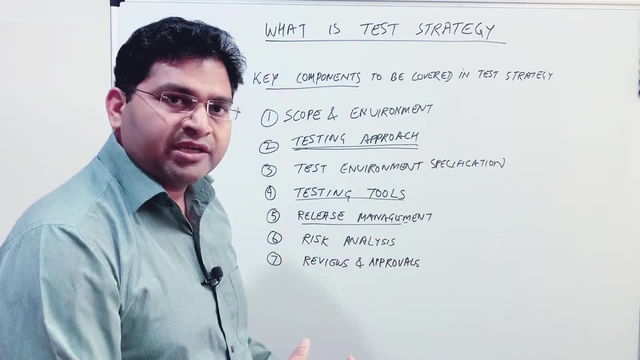 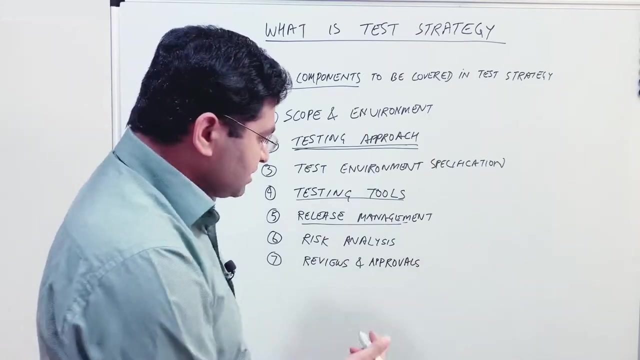 and project. a needs to be, you know, worked by uh, or reviewers can be, you know, like test test manager of the project, a project manager. so all those roles will go into uh, into the test strategy as reviews, reviewers and approvals and when any project is referring to the test strategy and 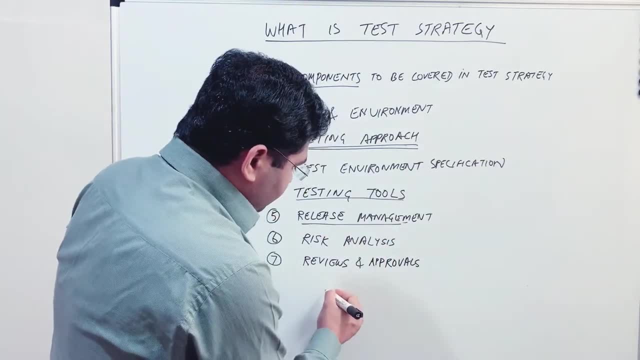 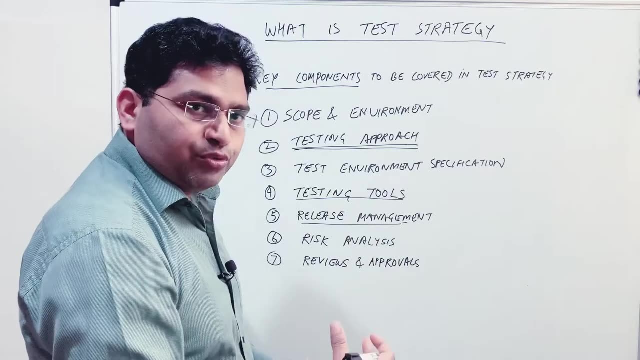 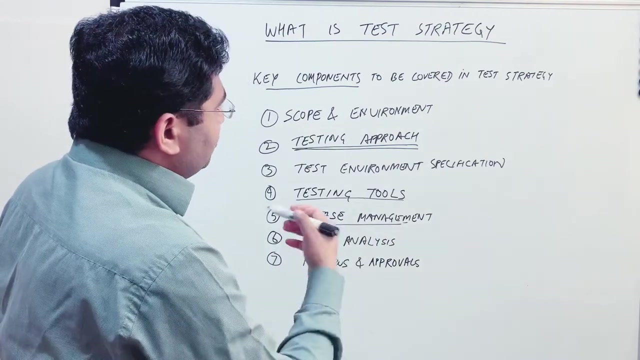 their own test plan. in that case, what they'll do is they'll refer to this section and in the test plan they'll mention those roles as reviewers and approvers for a particular project plan. okay, so these are the key sections that need to be included as part of the test strategy. 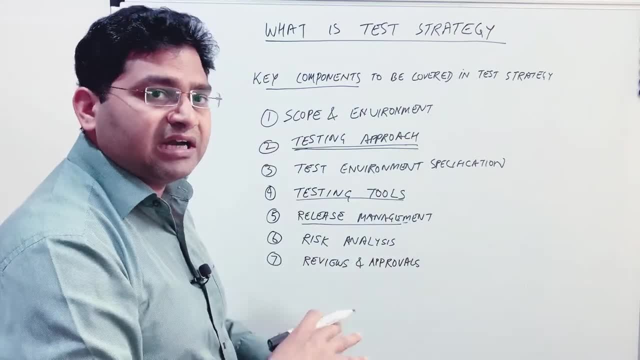 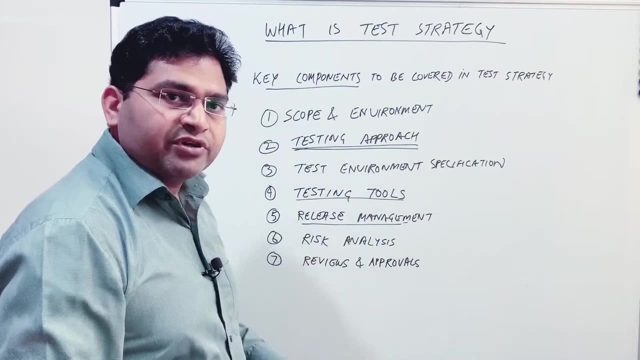 and test strategy is at the organization level, at the high level, and it defines all the information that a testing project needs to follow when a project is being tested, and it's a test strategy plan. so this is another section of the test plan where you will see everything: the test person. 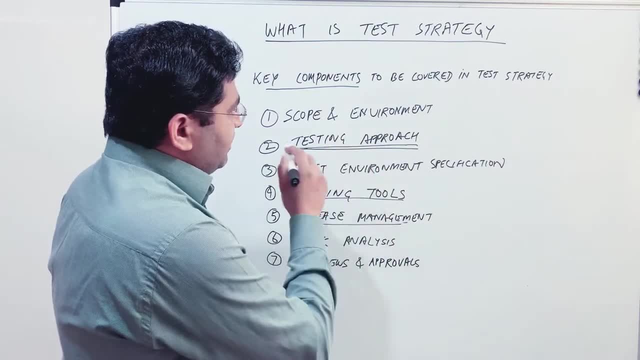 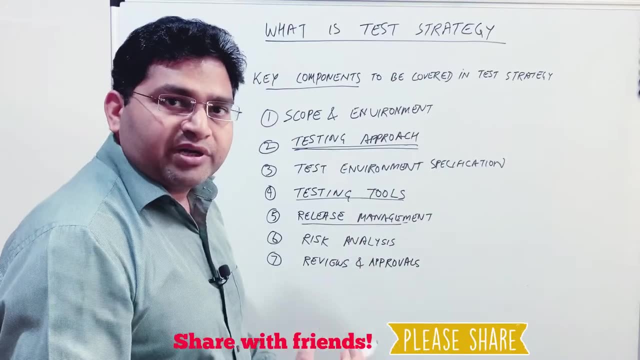 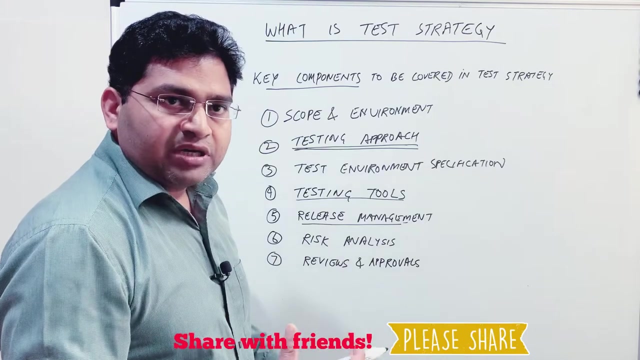 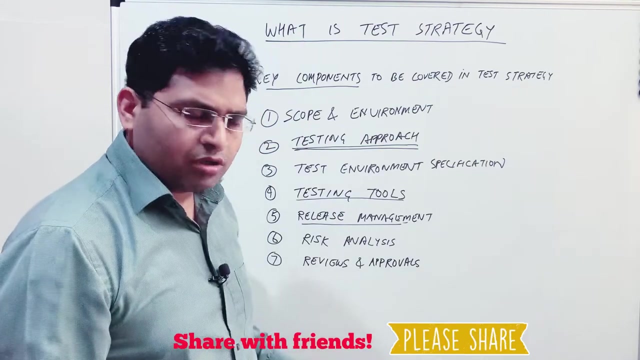 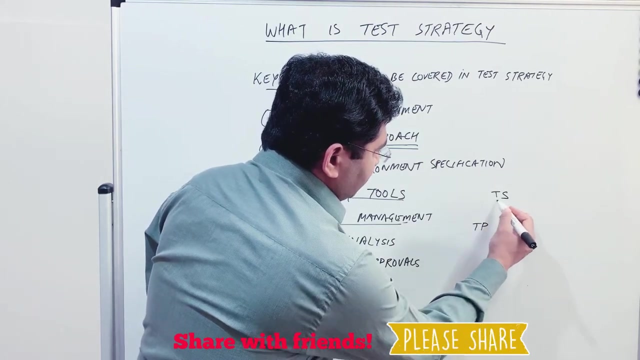 be used for testing the project and also이다ire taskwns that are a responsible Chore 연습. always program is always a test plan- go for review and so, in those case, the hierarchy of test strategy. so, for example, this is stress strategy and test plan. so, like it, the hierarchy is something like this for: 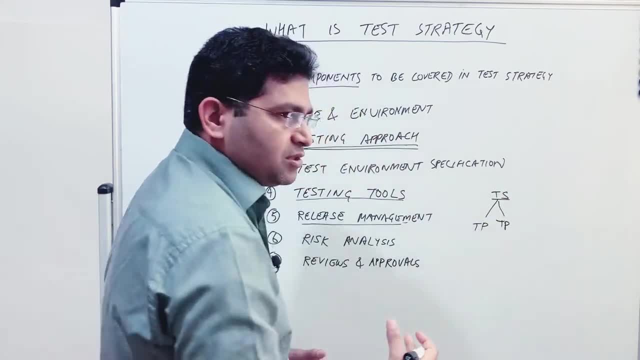 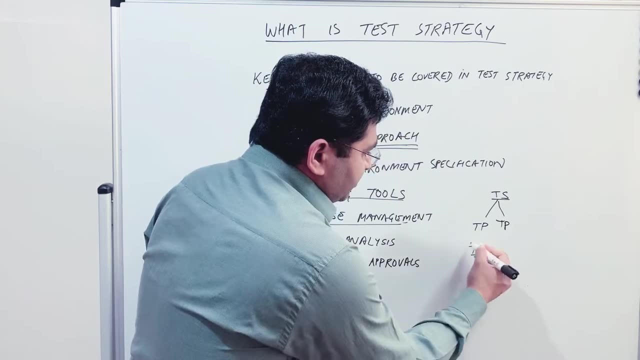 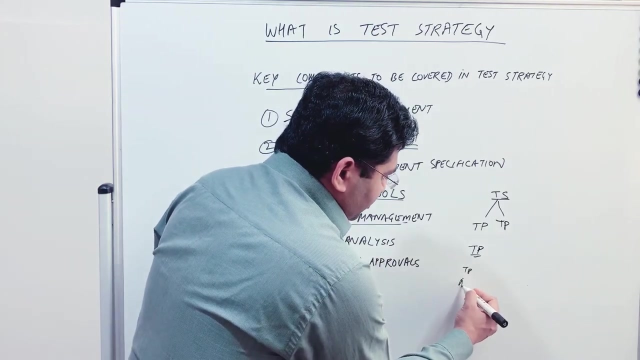 test strategy and test plan in big organizations, but in small organizations where you don't need there are, there are not many projects. in that case, within test plan itself the strategy or the test strategy will be elaborated right. otherwise in test plan during the approach or in the approach section. the 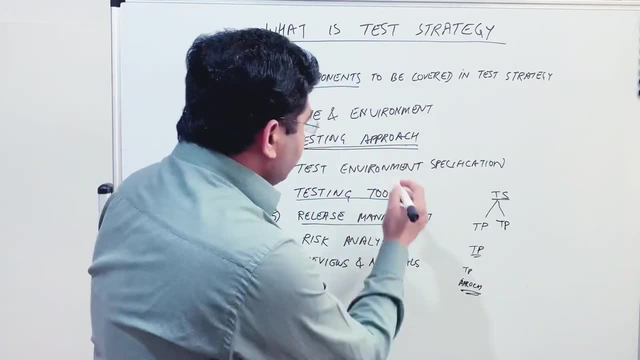 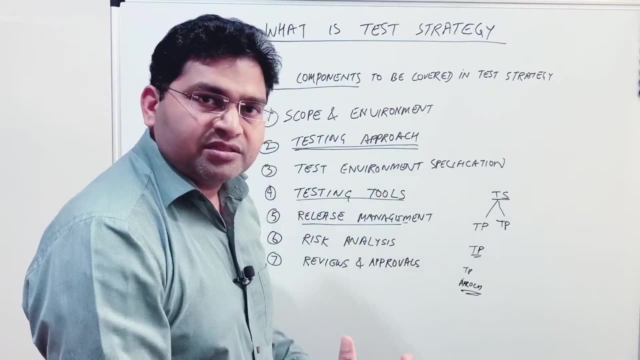 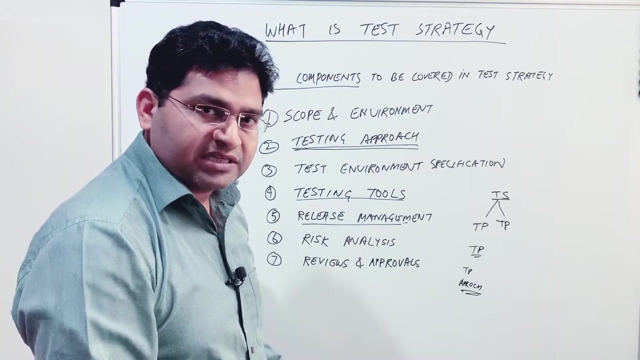 testing details or the test approach will be elaborated and you know testing approach from the test strategy will be applied and there will be more additions to that approach within the test plan. each test plan, each project as plan, as per the project details. alright, so that is all about the test strategy document. 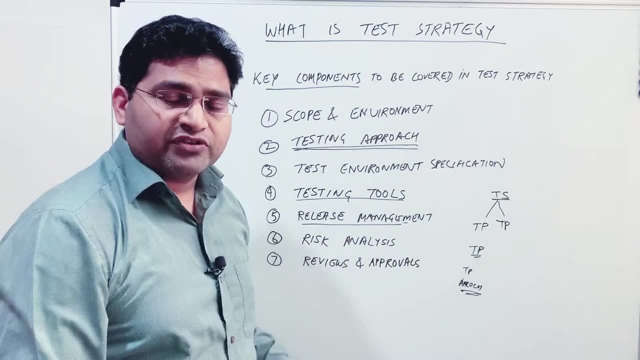 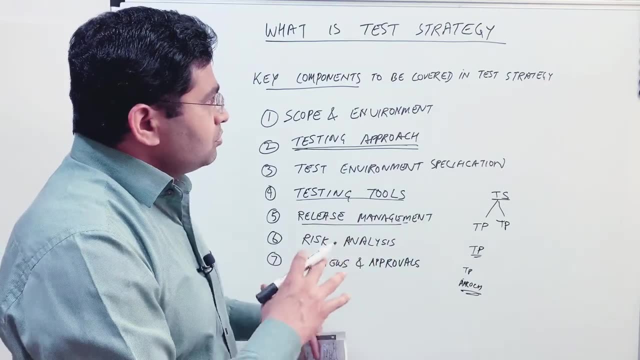 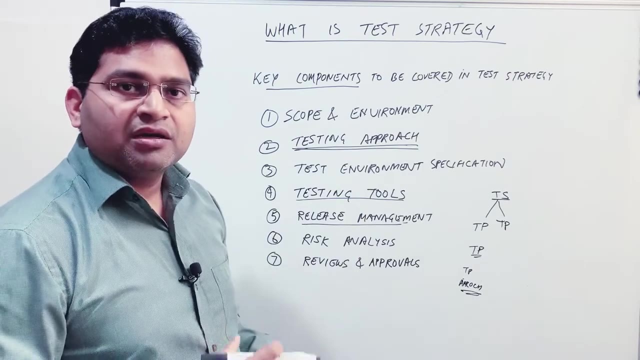 and why it is needed. test strategy is important and the hierarchy of test strategy okay. so i hope this was clear and you know. you are now clear about the test strategy and test plan relation. what exactly is test plan and how test plan how? what exactly is test strategy and how test plan is related to test? 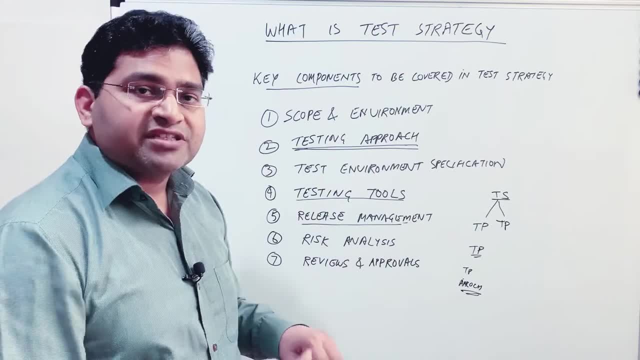 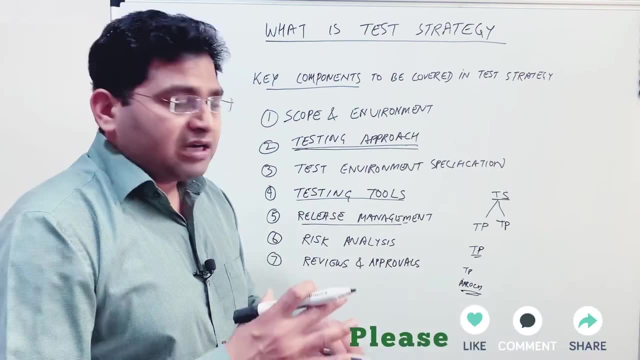 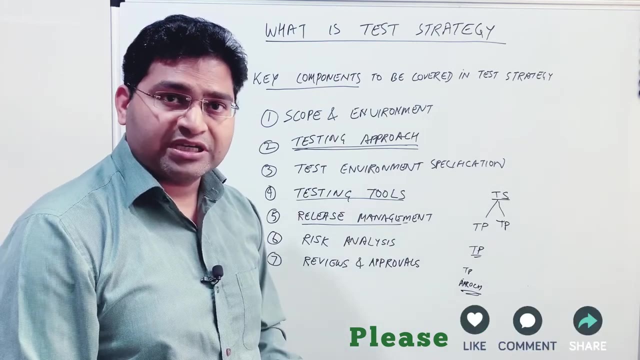 strategy and you know different options when test strategy will be written and when it will be part of the test plan. so in the next tutorial i'll cover the differences between the test strategy and test plan. so that's all for this tutorial. hope it was clear. please do share and subscribe, and thank you very much for watching.